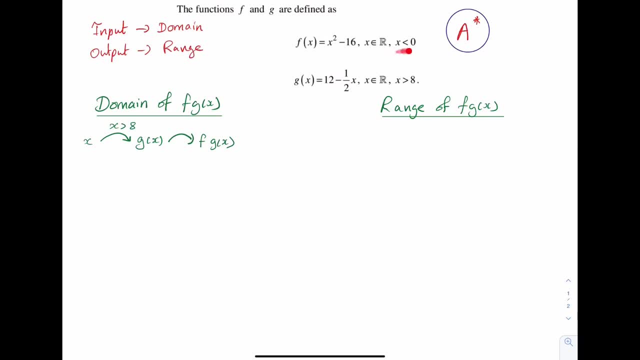 The input of f has to satisfy: x is less than 0.. G of x is our input for f. hence we must have that g of x is less than 0. So x is greater than single, So x has to be greater than 8 and g of x has to be less than 0. Now g of x is 12. 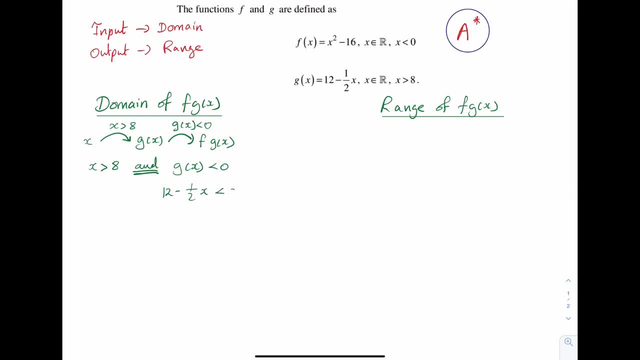 minus a half x, which has to be less than 0. I can go ahead and solve this particular inequality, So the first step will give me: minus a half. x is less than minus 12.. Therefore, x has to be bigger than 24.. So x is greater than 8 and x is. 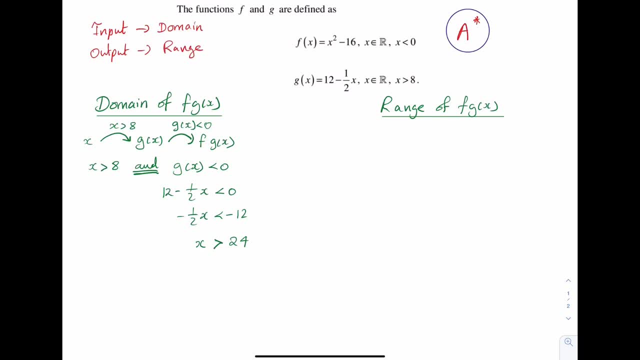 greater than 24.. The overlap is therefore: x is greater than 24.. So x is greater than 24. represents the domain of f, of g, of x. You can also include x is an element of the real number set. So I've got the domain of f, of g, of x. Now to find the range of f of 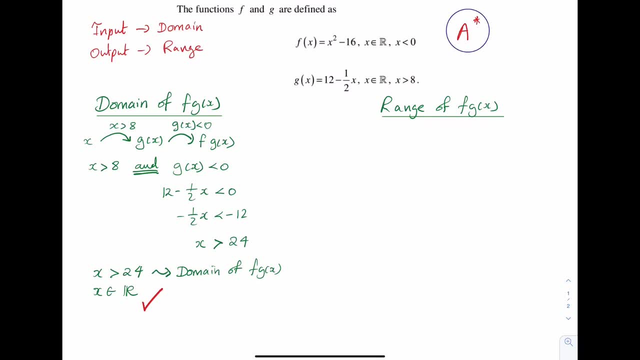 g of x. I'm going to sketch f of g of x for its restricted domain. Before I sketch f of g of x for its restricted domain, I'm going to first find the equation for f of g of x. f of G of x is the same as writing f in square brackets, g of x. So g of x is the. 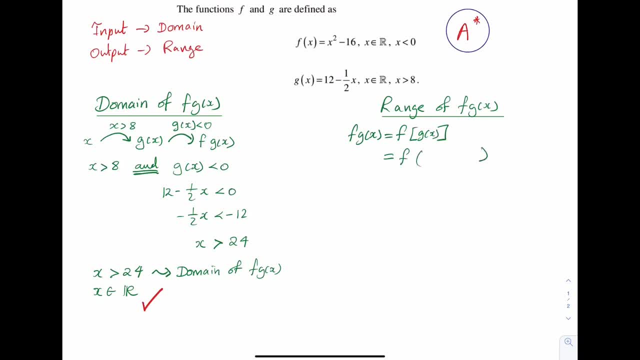 input. so I can write f in brackets: 12 minus a half x. So if I replace the x in f with 12 minus a half x, I get the following result: 12 minus a half x in brackets, squared minus 16.. Now we can make two observations. This particular quadratic will be a positive.